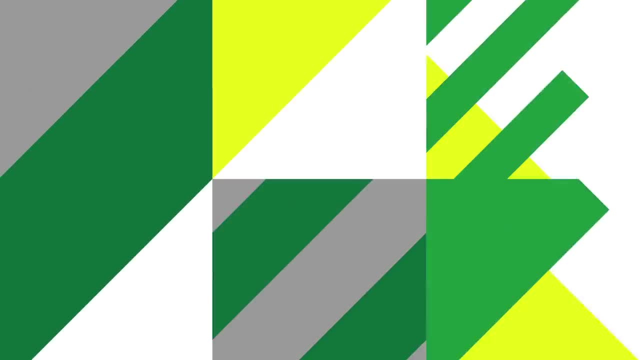 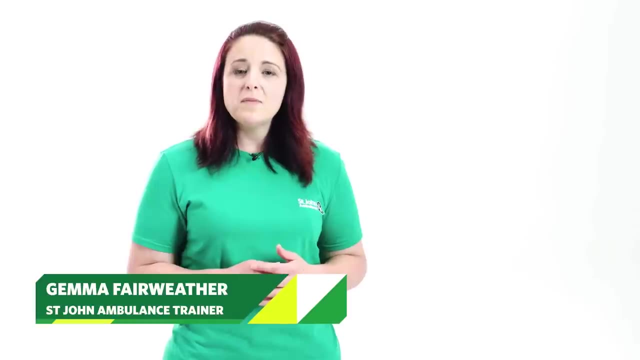 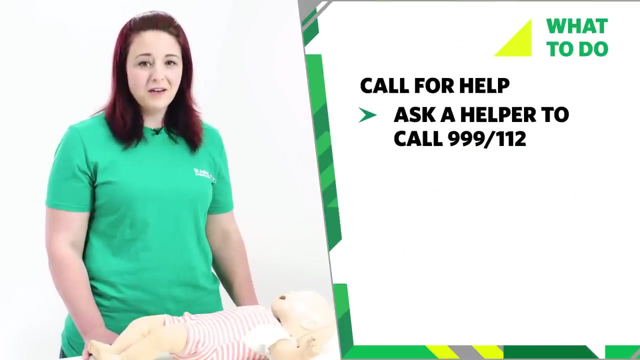 If you ever find your baby is not responding to you, you will give them the best chance of survival if you know what to do. If you have found your baby unresponsive and not breathing normally, you will need to perform baby CPR. Call for help. Ask a helper to call 999 or 112 for emergency help. Use a mobile speaker. 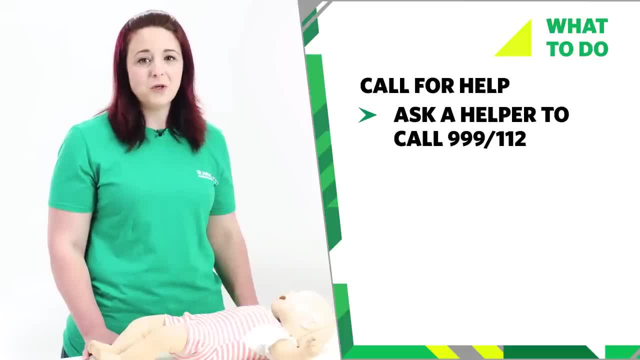 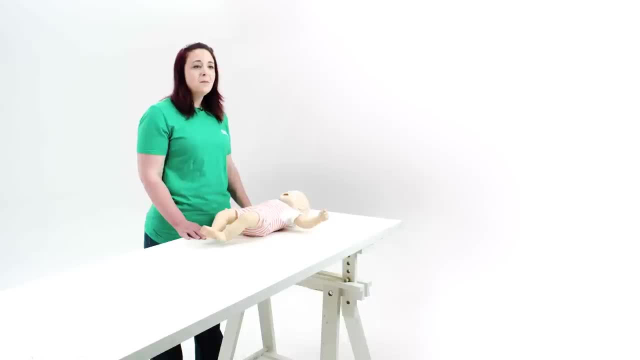 phone if you're on your own, so you can start CPR as soon as possible. If you're on your own and you don't have a speaker phone, you need to do CPR for a minute before you can call for help. Place them on a firm surface and open their airway With one hand on the 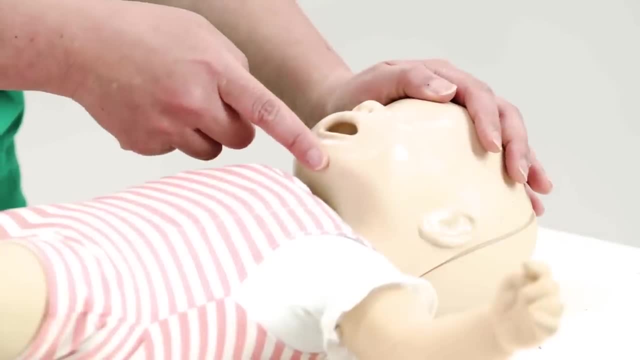 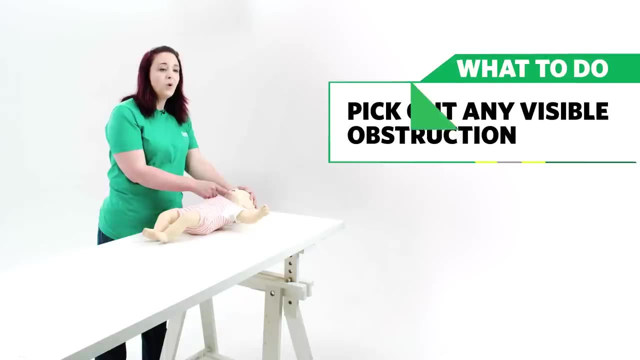 forehead. gently tilt their head back With your fingertip. gently lift the chin to open the airway. Pick out any visible obstructions from the mouth and nose. Step one is Puff. Take a breath, put your lips around your baby's. 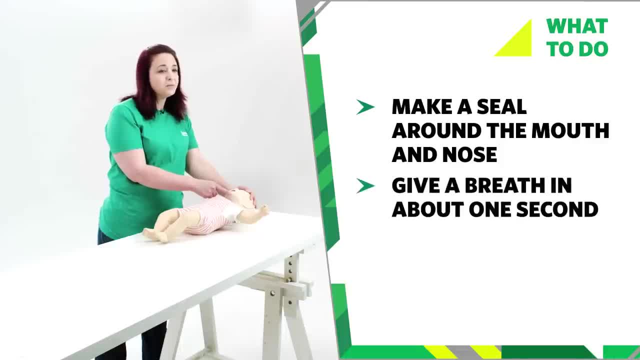 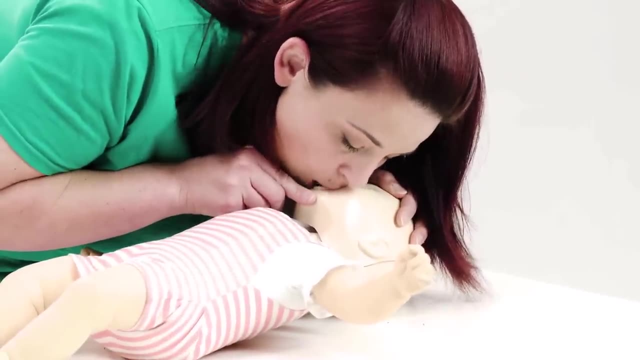 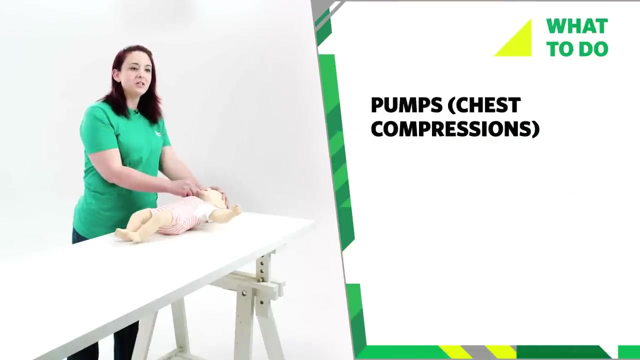 mouth and nose and make a seal. Blow gently and steadily for up to one second. The chest should rise. Remove your mouth and watch the chest fall. That's one rescue breath or puff. Do this five times. Step two is Pump or chest compressions. Put two fingers in the centre of your baby's chest. 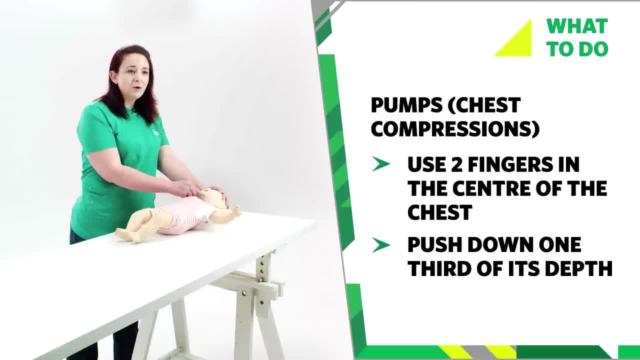 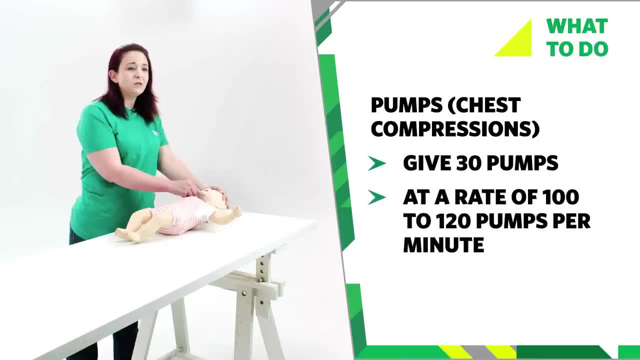 and push down a third of the depth of the chest. Release the pressure, allowing the chest to come back up, before pressing back down again. Repeat this 30 times at a rate of 100 to 120 pumps per minute. This is quite quick. 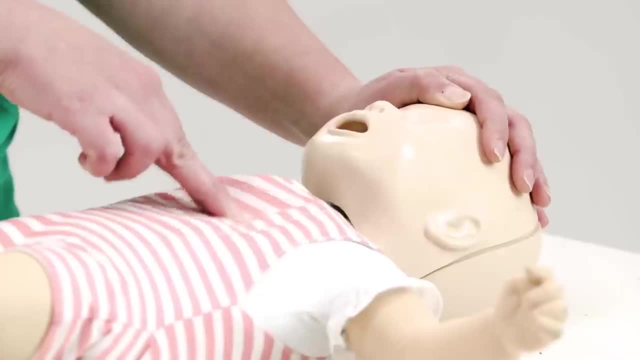 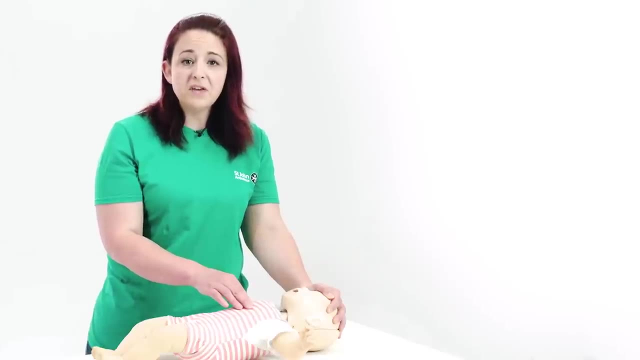 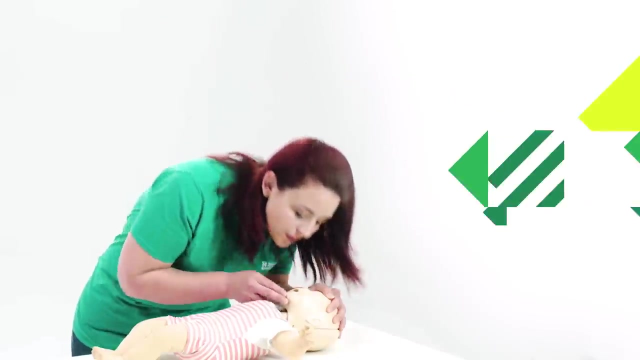 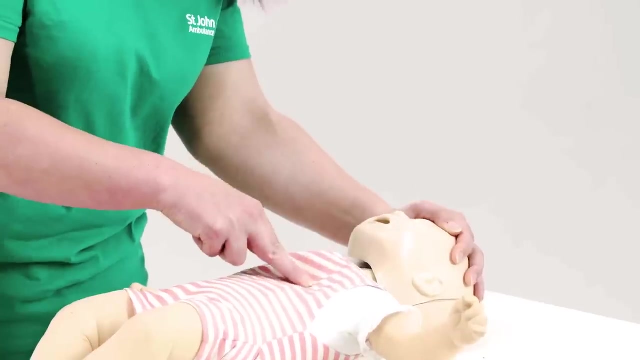 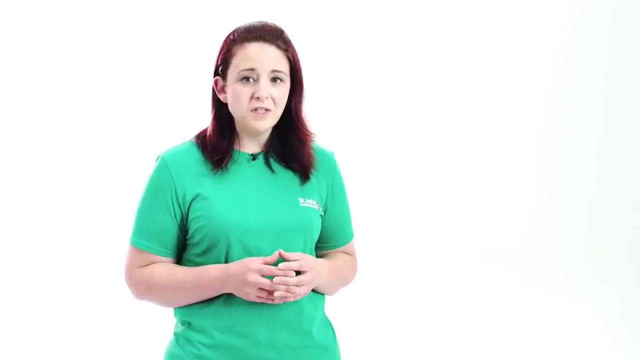 After 30 chest pumps, open the airway and give a further two puffs. Continue to alternate between 30 chest pumps and two puffs. If you're on your own and don't have a speakerphone, stop after one minute and call 999 or 112 for